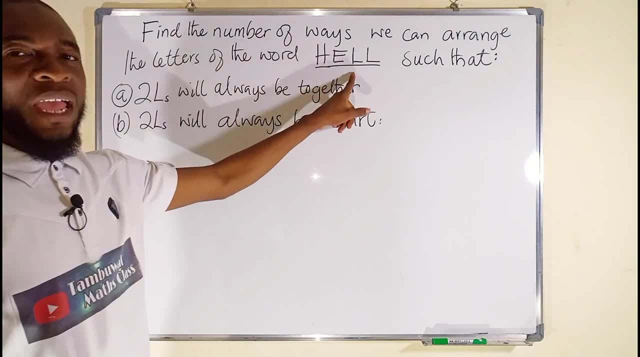 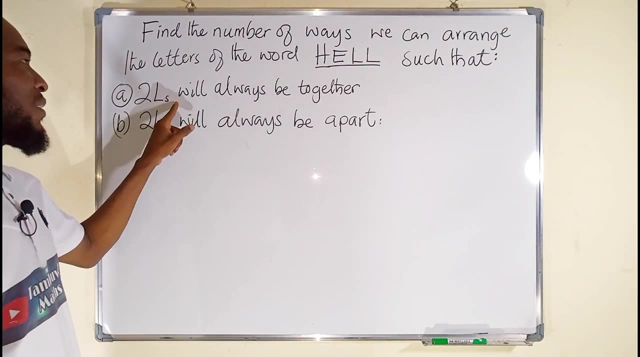 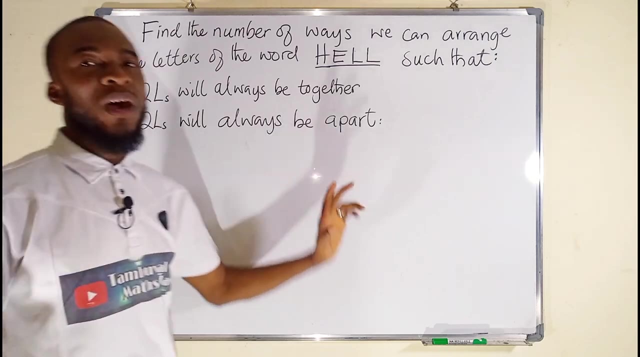 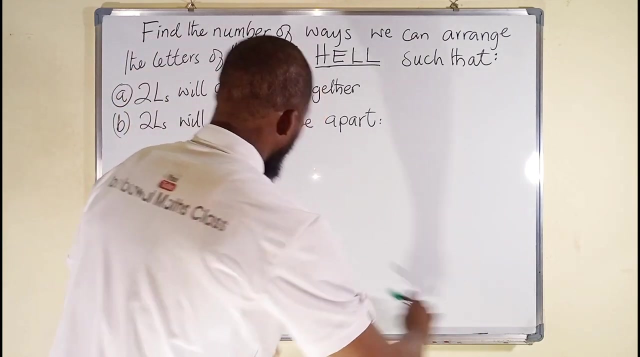 arrange the letters of the word hell such that- this is the condition Number one- two L's will always be together. Second condition is that two L's will always be apart. Let's start with the first one. in the case where the two L's will always be together, So a part, the word is: 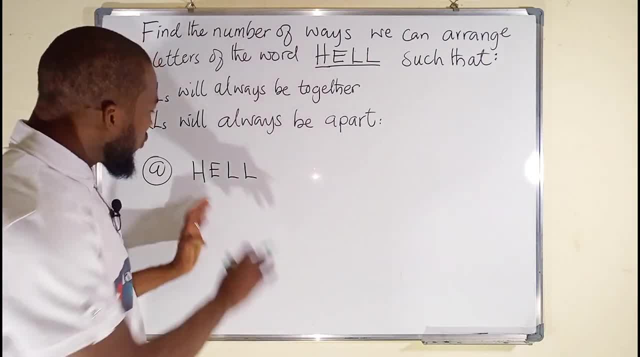 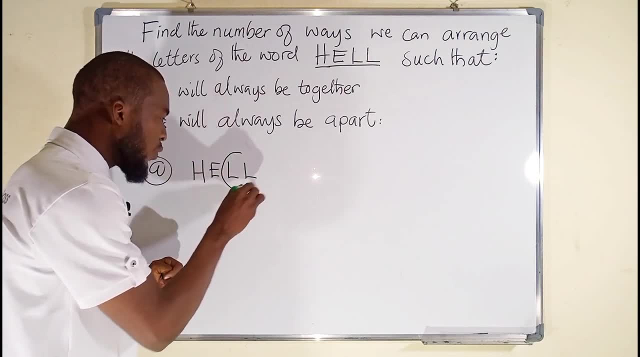 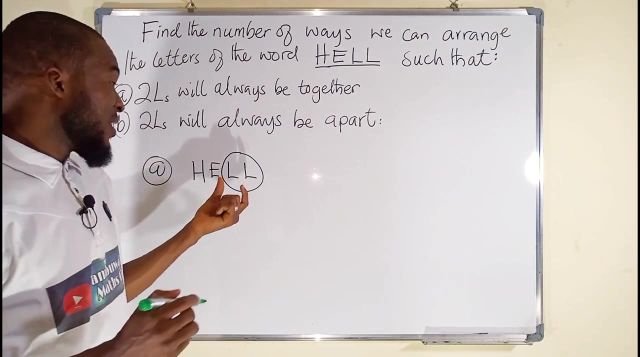 hell. We want to arrange this word, or the letters of this word hell, in such a way that the two L's will always be together, So, no matter where you shift it- it could be here, here or here- This means that it is going to be treated as a single letter, And hence we have one, two, three And. 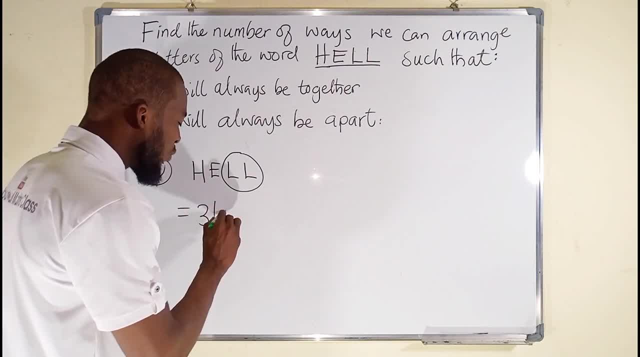 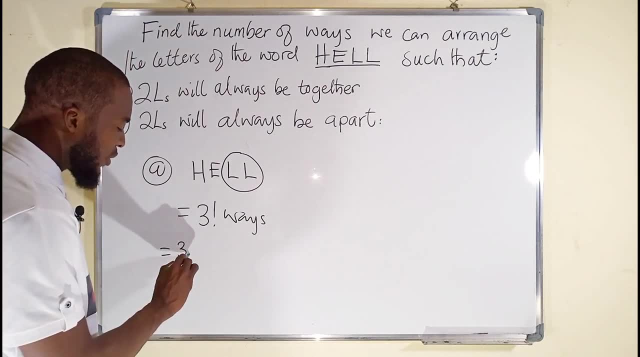 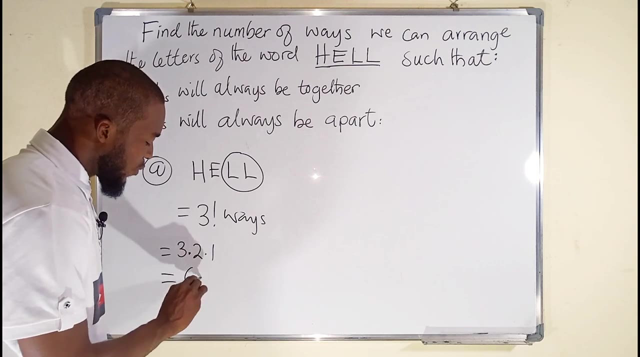 this is equal to three factorial ways, And three factorial, remember, is the same thing as three multiplied by two, multiplied by one, And this is equal to three times two. six times one is six. So we have six different ways in which we 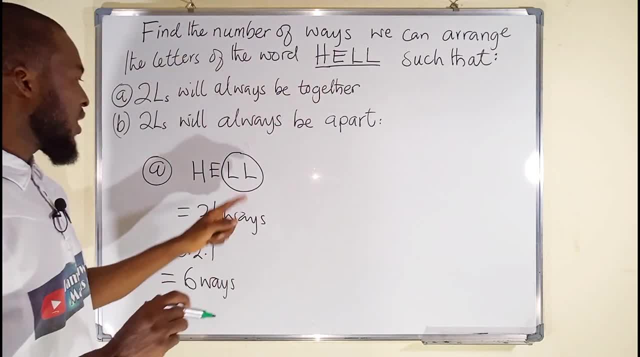 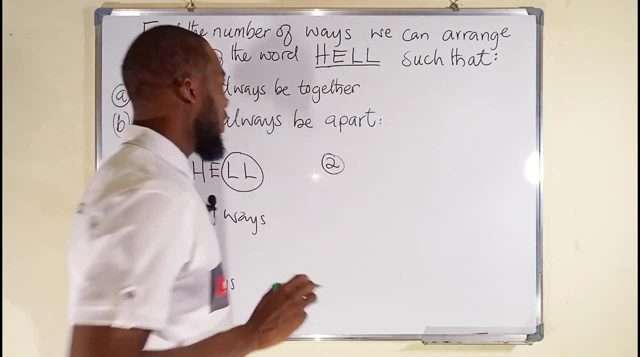 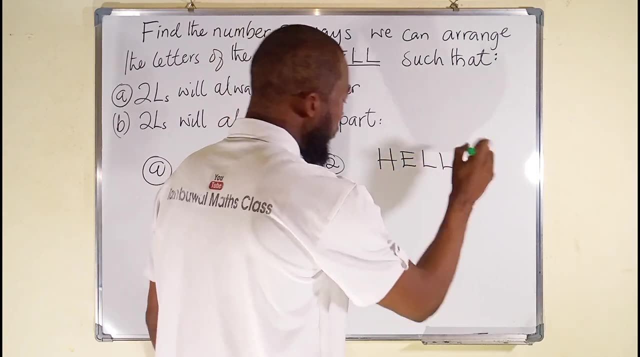 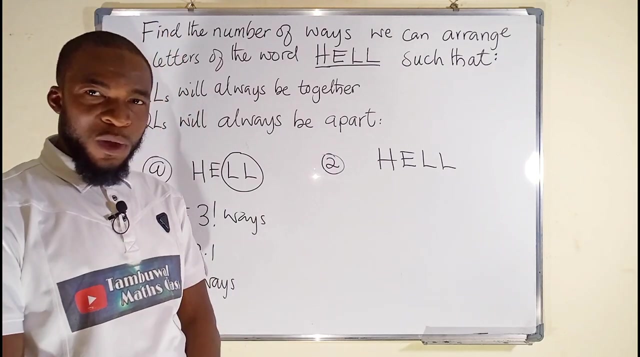 can arrange the letters of the word hell such that the two L's will always be together. Now let us talk about number two. Number two: we still have the same letters- hell, But this time around we don't want these letters to be together. So how can we do that If we don't? 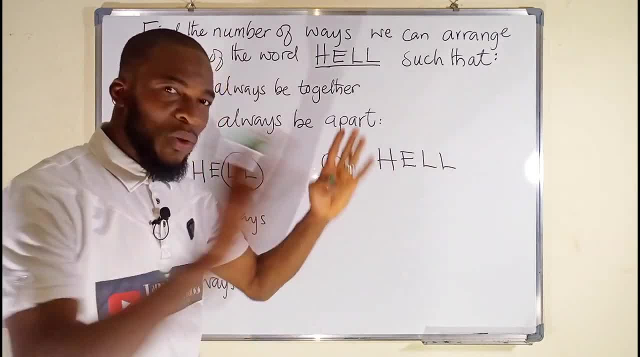 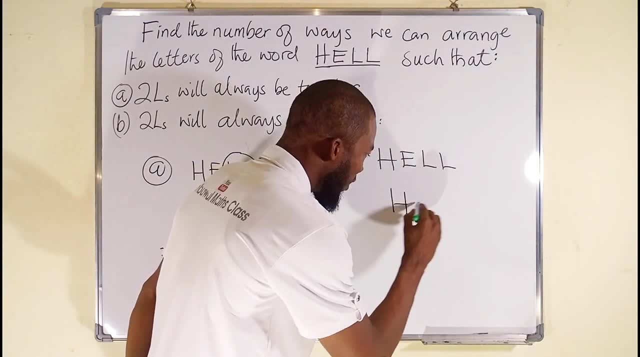 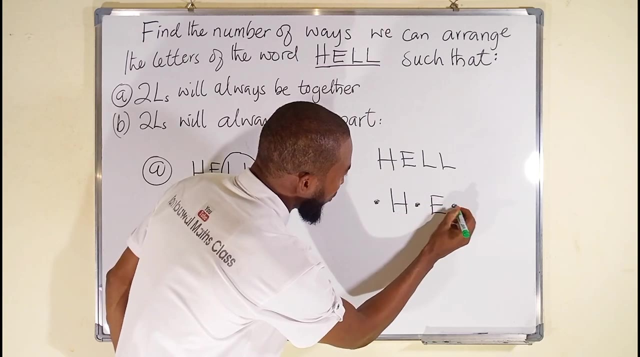 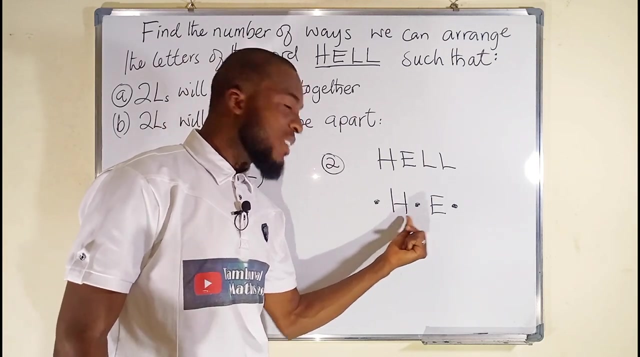 want these to be together. therefore they have to be in between or side by side of the letters H-E. So if we have the letters H here and E here, this L's could either be here, here or here. But we know that we have two factorial different ways of arranging H-E, So we don't have 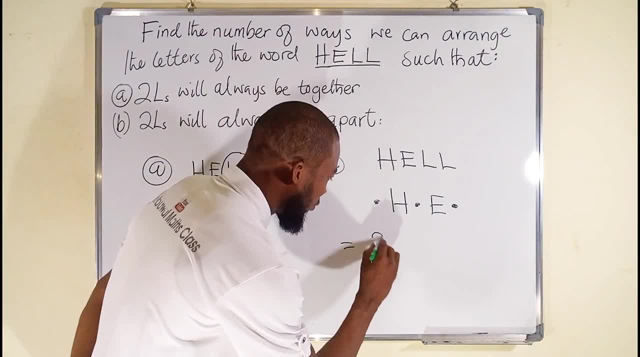 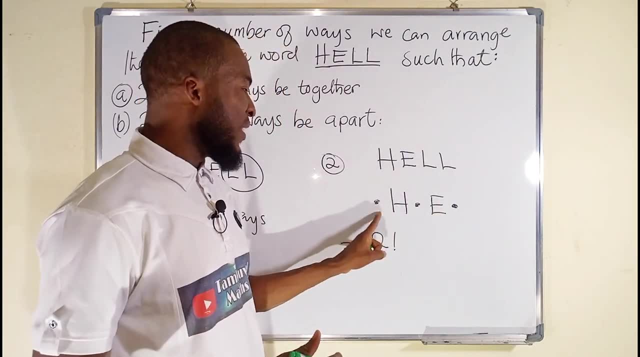 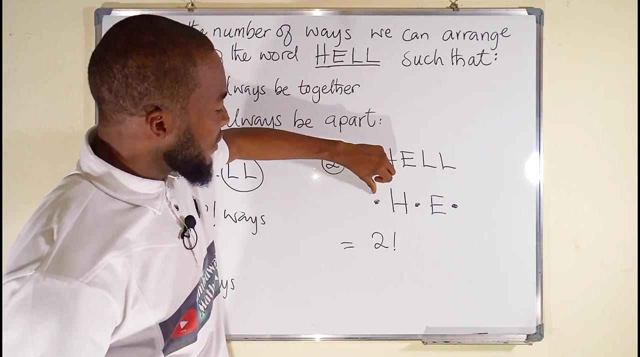 a problem with that one. I can even write it. This is the same thing as two factorial And we have to find out how many ways we can arrange the letters LL such that it fits these positions. OK, suppose this is our first L and this is the second L. You can fix this first L here and the second L.